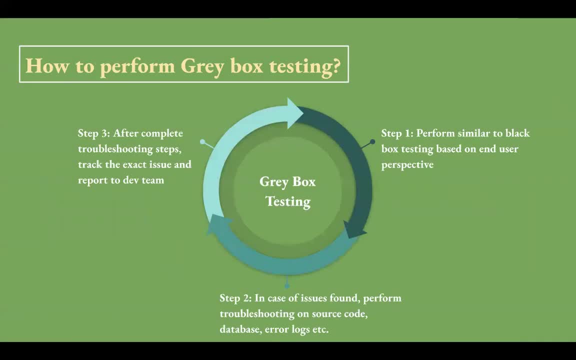 Let's discuss how to perform grey box testing. Normally the testing is performed as per user perspective, Then black box testing, But if there is a requirement that test cases should be created based on the exact workflow implemented in the code, then the testers can refer to project. 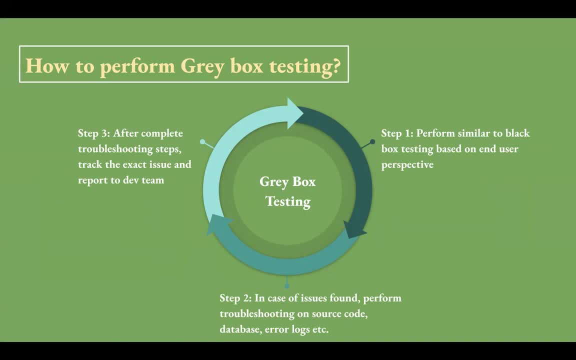 code and internal design structure of project. If there is a need, only then we can refer to source code which can help in creating more test scenarios on that particular feature to find more defects. But in white box testing the testing is performed based on the logical part of code. 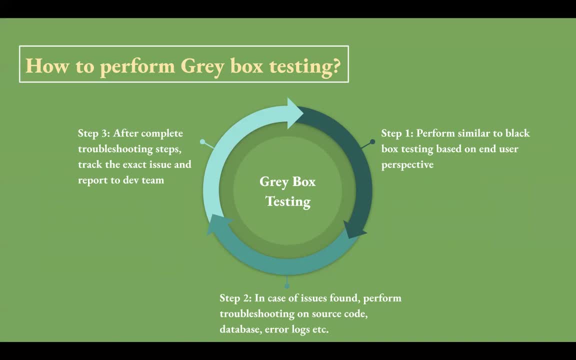 In grey box testing. the testing is fully performed based on source code In grey box testing. at first step, you will perform testing similar to black box in which you will execute your test cases on behalf of end user, like how end user will interact. 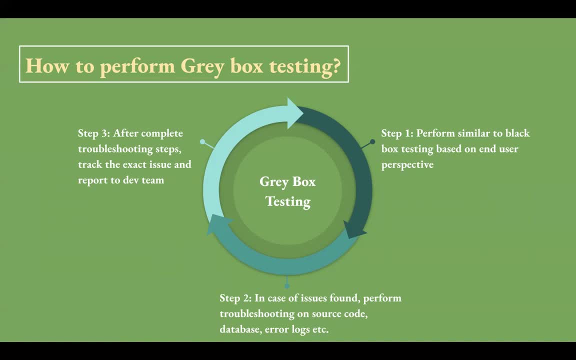 with that application And during that process, suppose you found any issue. Now you will confirm that, whether that issue appears in the application or not. If that issue appears at functionality level then that can be resolved without troubleshooting further in the source code. But in case you found that scenario is not handled by the 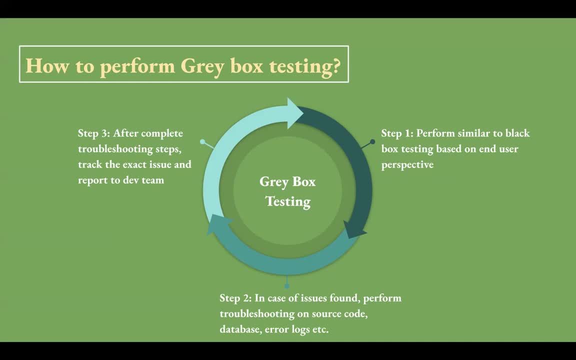 developer and you need to reconfirm before raising the bug. Then for troubleshooting purpose you have to check the source code. The test cases could be related to UI, database or any operation performed. So this is one basic example. Another example would be that suppose you opened any page of website and your website 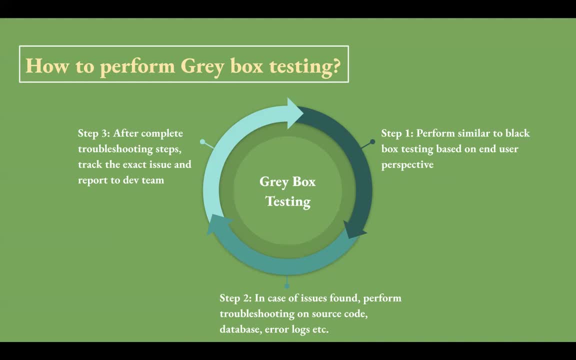 page is not loading and you get some error code. So to troubleshoot further, you can check the logs of that website. So in that case you should have little bit knowledge of where all logs are getting stored. And suppose you are performing testing on APIs and your API is not responding as per. 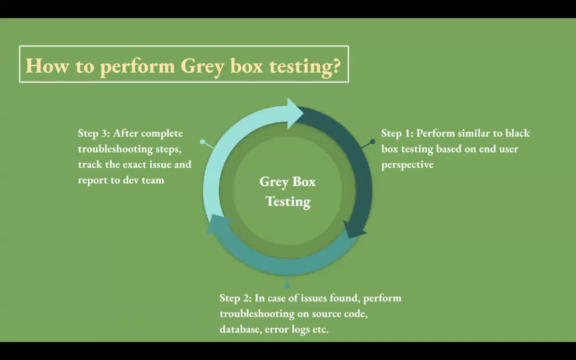 the expectation. So if you have access to source code and database access, then you can troubleshoot and confirm where is the exact issue and you can directly report that issue to development team for fix. So little bit of knowledge regarding source code, database, error logs etc. will be helpful.